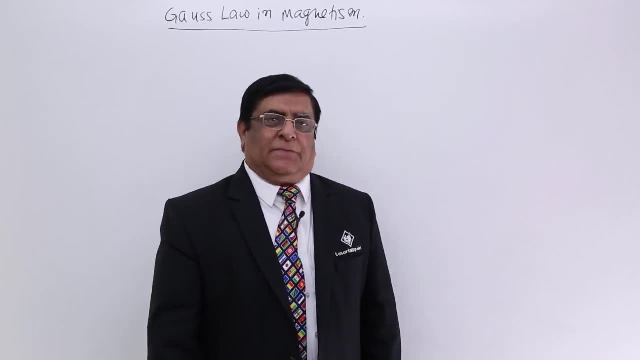 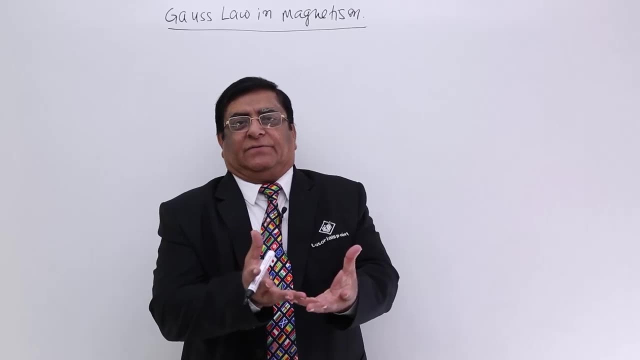 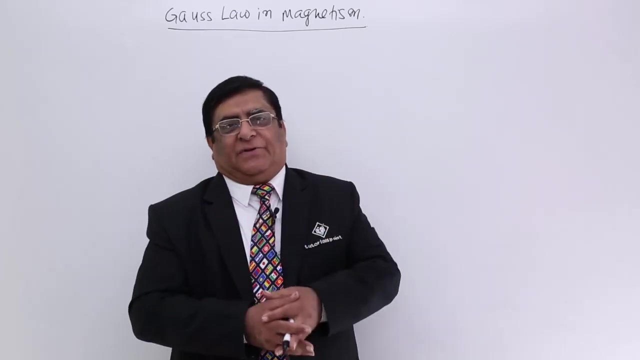 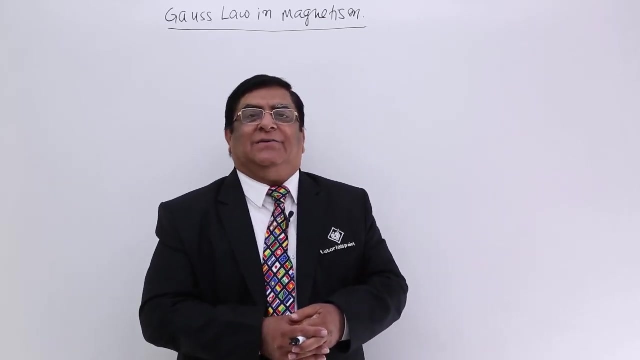 We had a Gauss law in electrostatics. The Gauss law deals with a surface which encloses something In electricity. in electrostatics it used to enclose an electric field. Here we will consider a surface which is spread in a magnetic field. So if it is a closed, 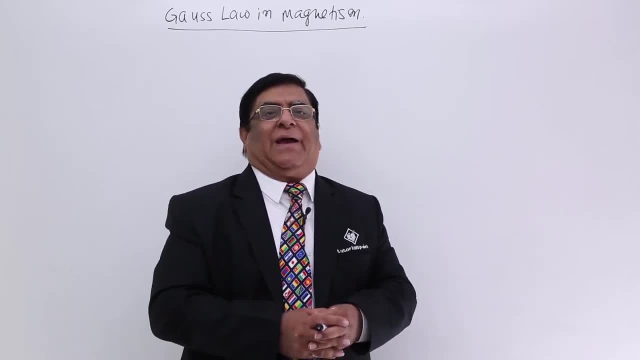 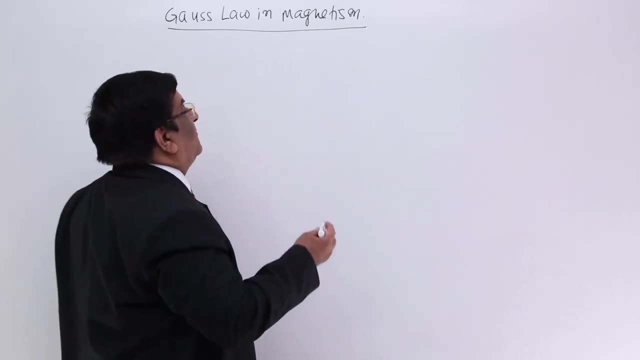 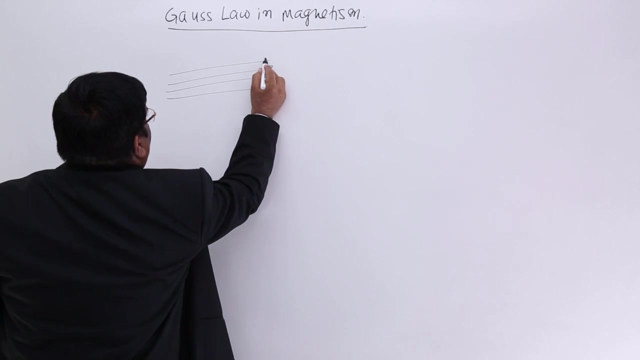 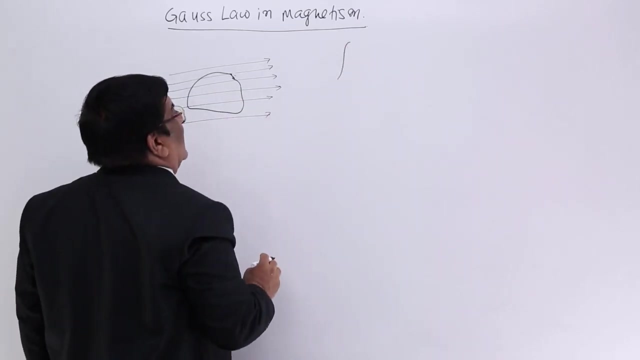 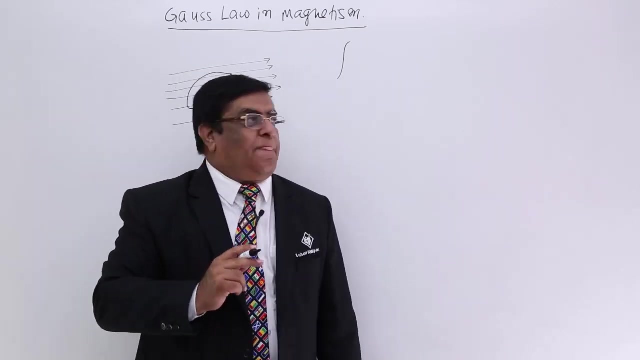 surface, then closed surface in magnetic field will be touching magnetic field at each and every point. And if there is a magnetic field 1 a surface, then it is a closed surface and the total magnetic flux- here we are introducing a new word, that is magnetic flux. 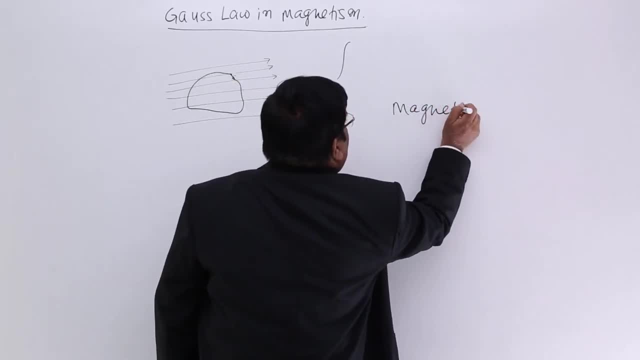 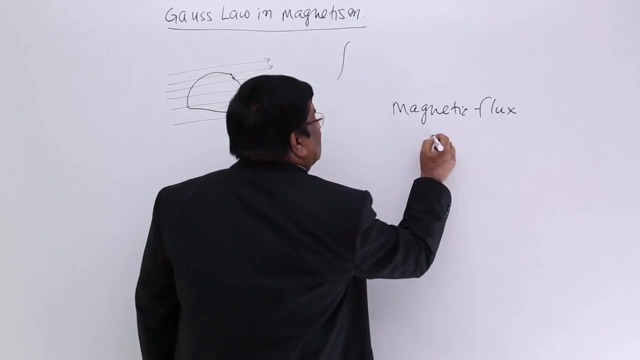 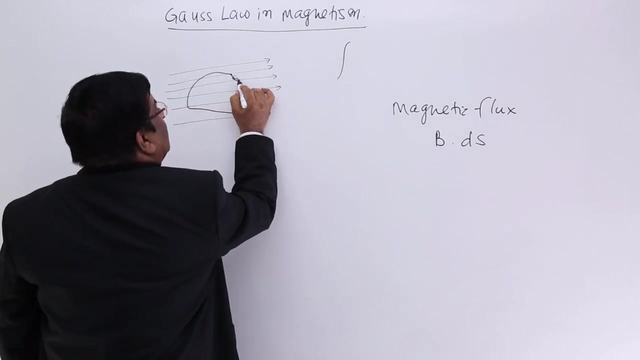 Magnetic flux is just like electrical flux or electrostatic flux, that is intensity of the field multiplied by the area it is touching. So if we take a very small area here, ds, this is magnetic field. B, B multiplied by ds, that is B dot ds. 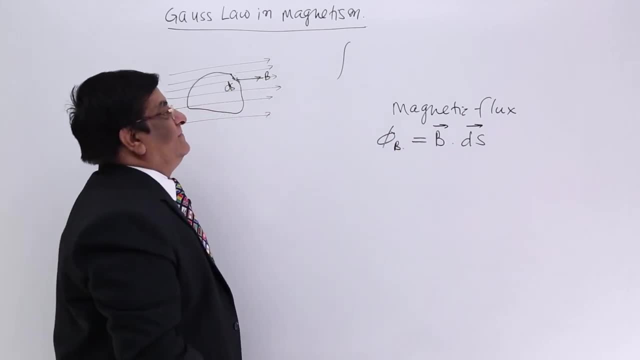 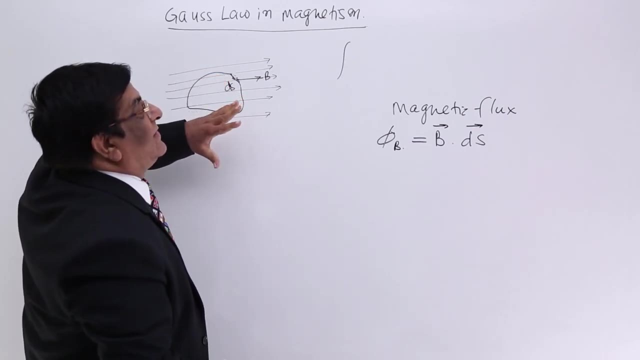 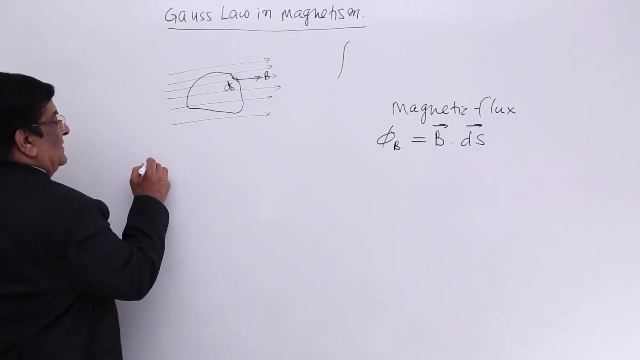 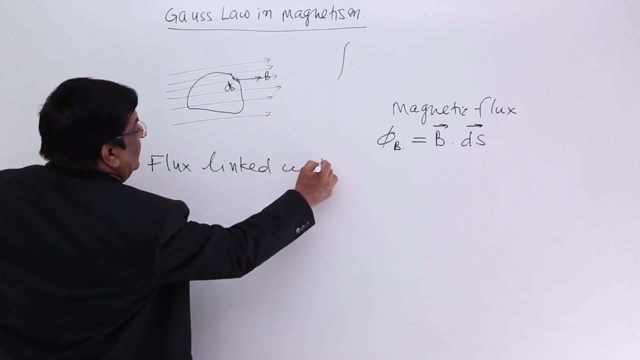 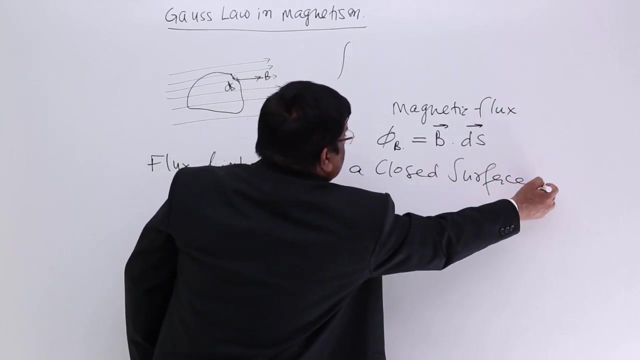 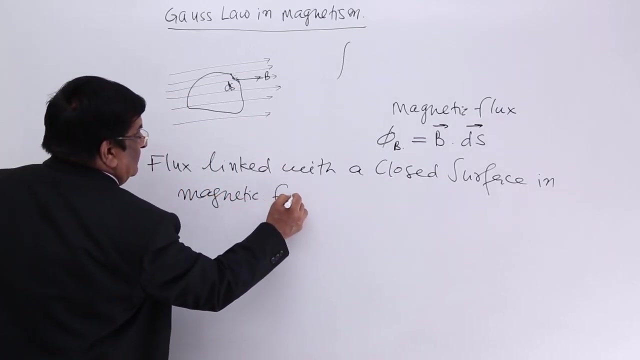 This is known as magnetic flux. Now, the total magnetic flux linked with the surface, how much is that? That is the Gauss law in magnetism. So Gauss law in magnetism, speak about what Flux linked with a closed surface In magnetic field is how much. 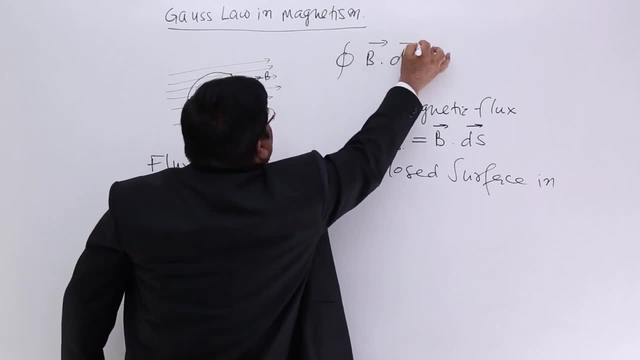 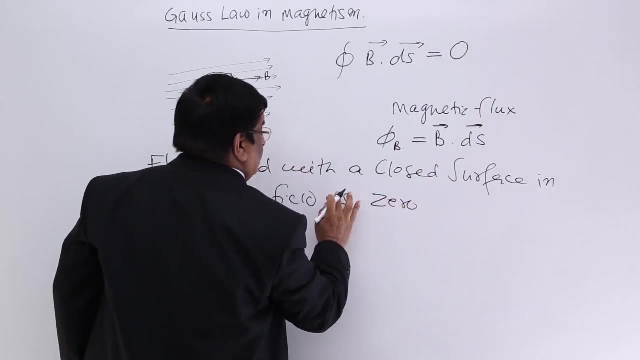 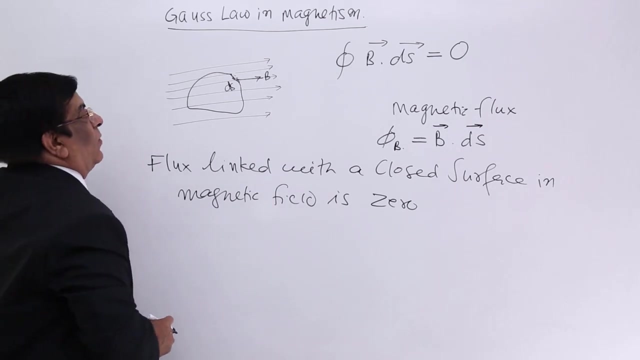 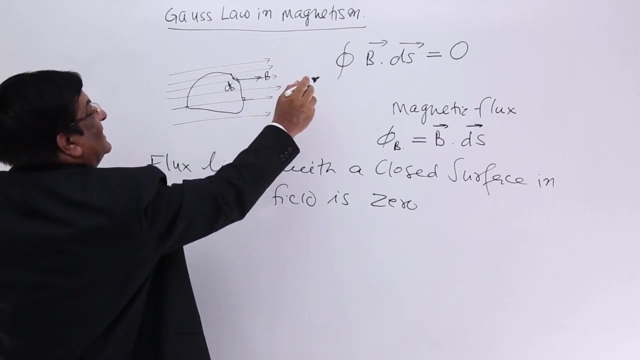 Closed. integral B ds is how much? Answer: this is zero. So this is Gauss law in magnetism. Thank you, Why? Answer is here, this is going out and here it is going in. So if we make the integration, then the total B ds. this at many places positive, at many. 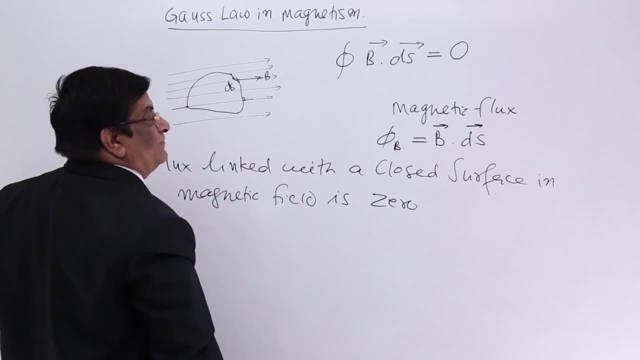 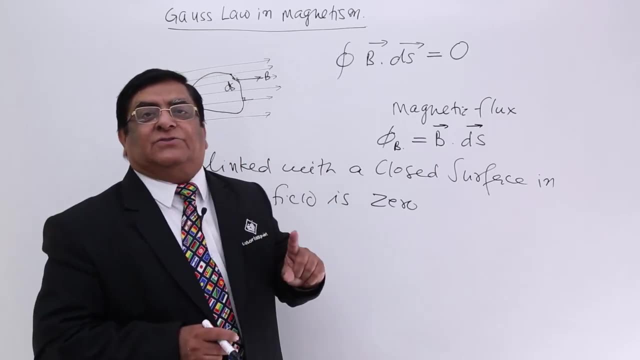 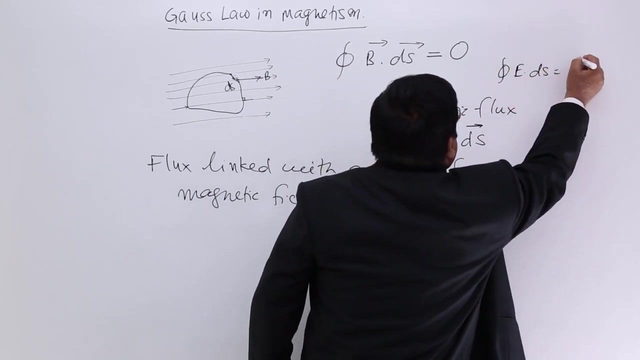 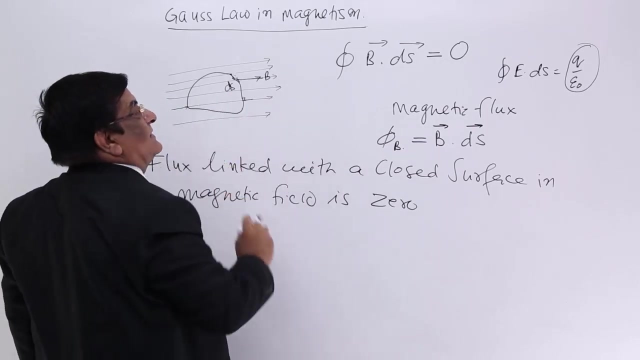 places negative and the sum will be zero. Is it always zero? Yes, it is always zero, And very unlike to electrostatic Electrostatic Gauss law, which used to say that closed integral E ds is equal to Q upon epsilon naught. It depends upon how much is the charge within the Gaussian surface. 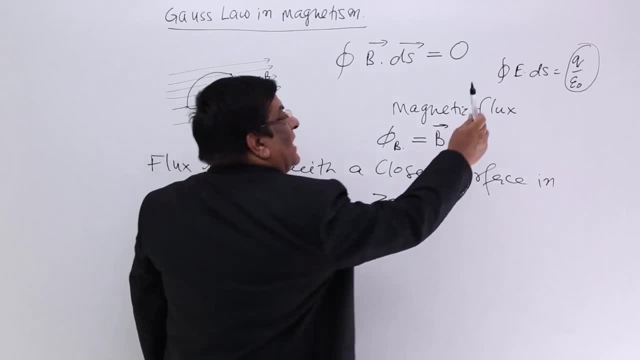 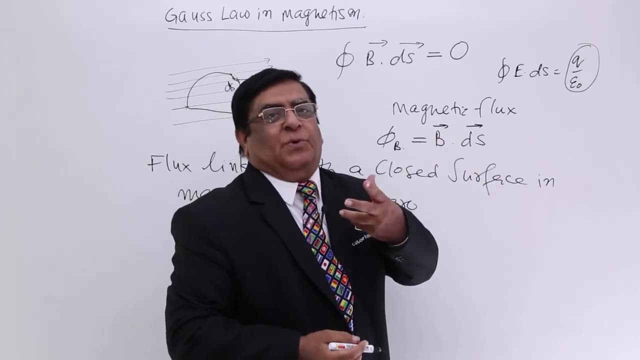 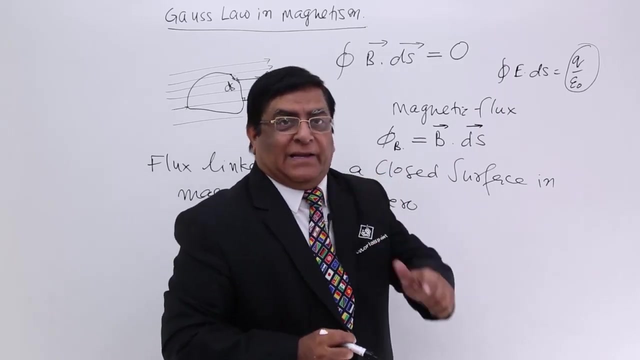 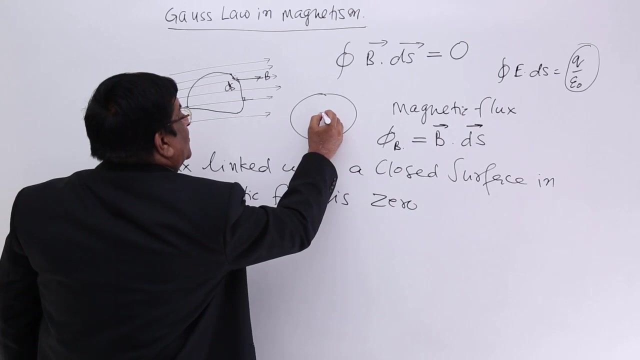 But here it is immaterial Charge is the one which is responsible to create electric field. Why, Who is responsible to create magnetic field? Answer: North Pole and South Pole in material magnetism. So if I take a Gaussian surface and I put a North Pole here, the answer is I have to put. 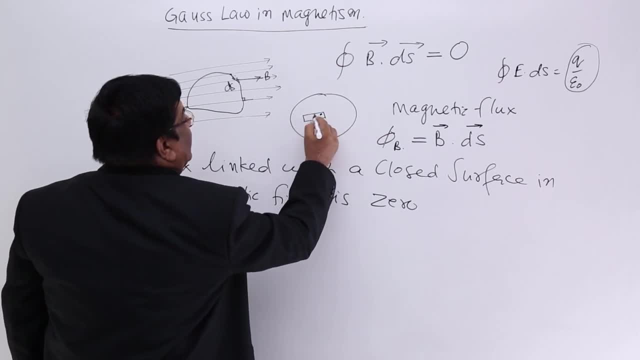 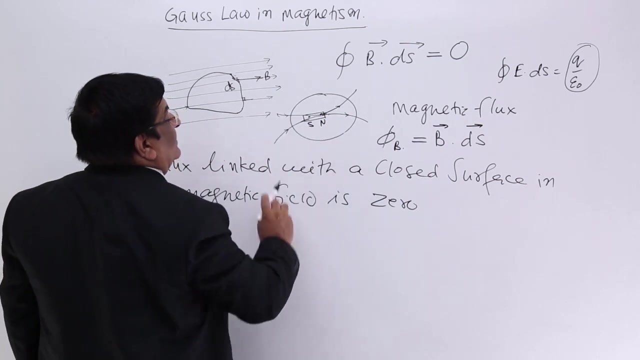 a magnet and North Pole and South Pole cannot be separated. So a South Pole is also here Now from North Pole the magnetic field lines go out. From North Pole the magnetic field lines go out From South Pole, they enter. So the number of lines which are going out are equal to number of lines which are entering. 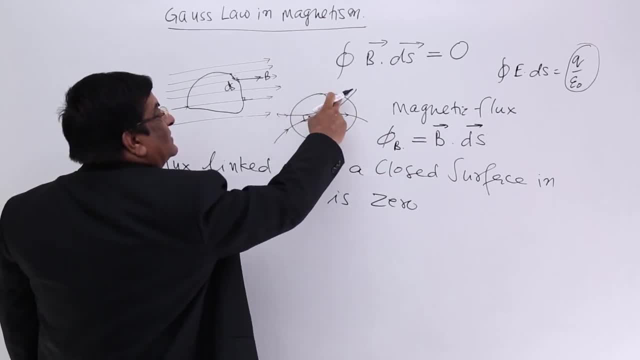 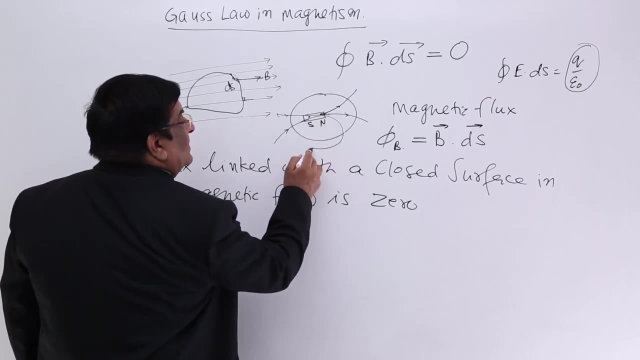 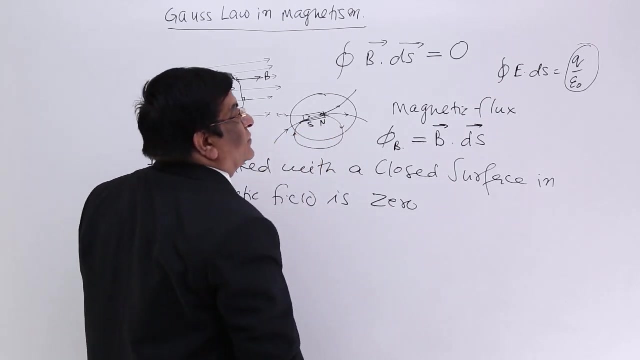 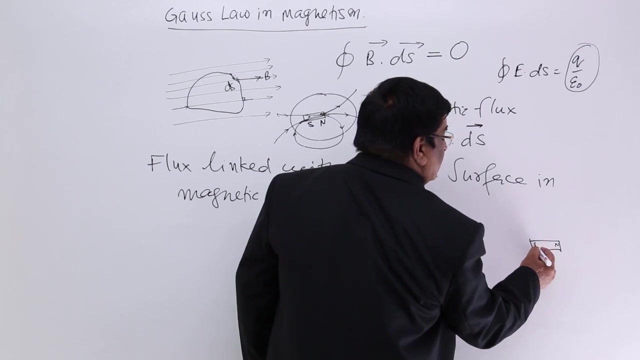 So the total number of lines with the closed surface is zero. The total effect is zero because the number of lines going out are equal to number of lines entering. in this way, So this is the solution, Thank you, Thank you. So now, in a bar magnet we cannot separate the two. if we cut it here we have a South. 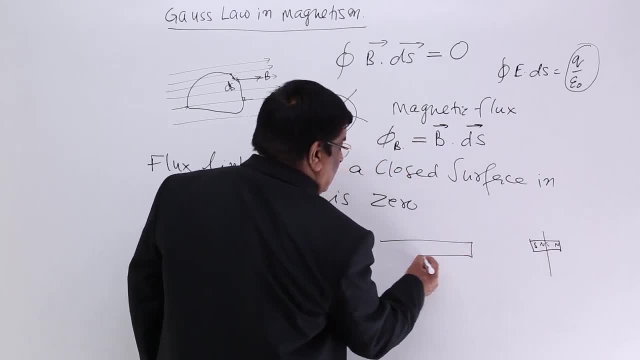 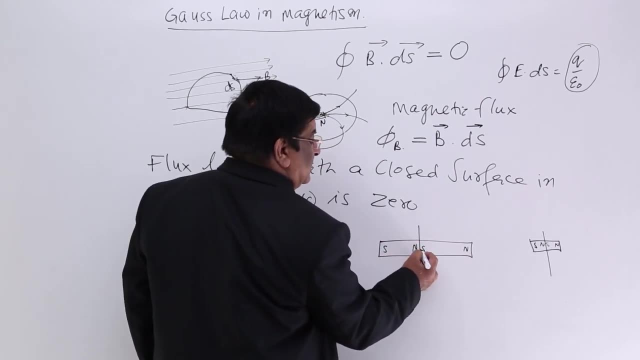 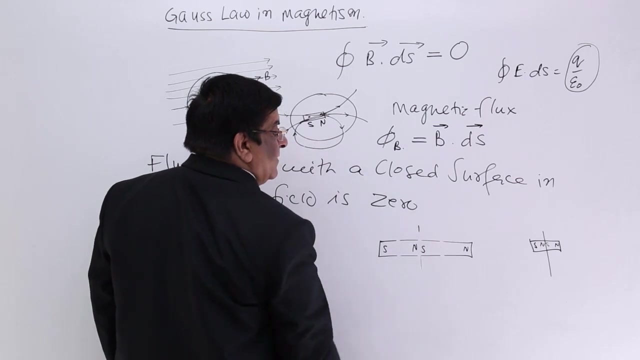 Pole here. We have a North Pole here. Cut it. We get a North here and a South here. Now, if we cut it here, Then what will happen? Answer: we get a south pole here and we get a north pole here. 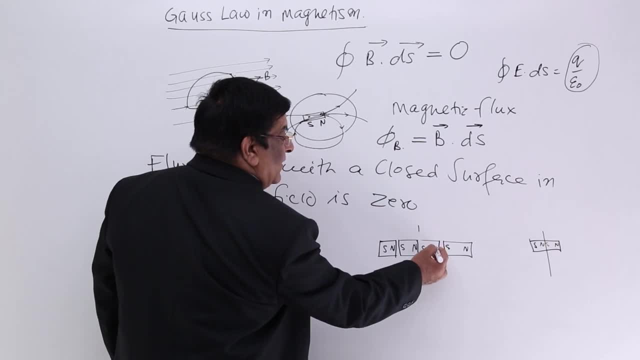 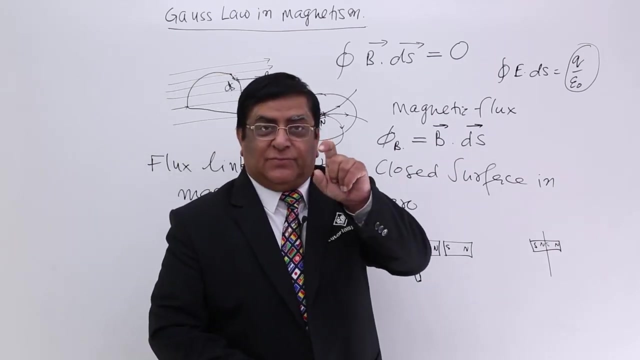 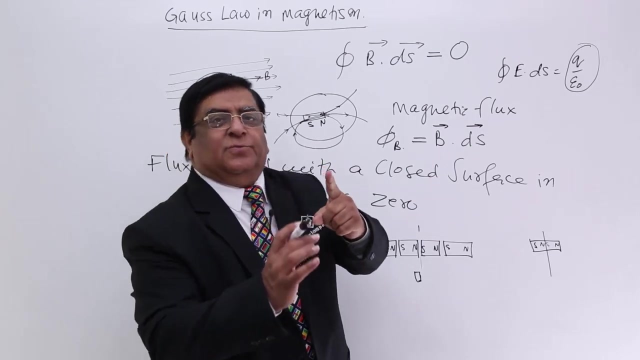 You cut it this way, you get a south pole here and a north pole here. In this way, whatever small cut you made, any small particle, even if it is a single electron. you cannot cut that. Even if a single electron is rotating this way, from one side, it is north pole from. 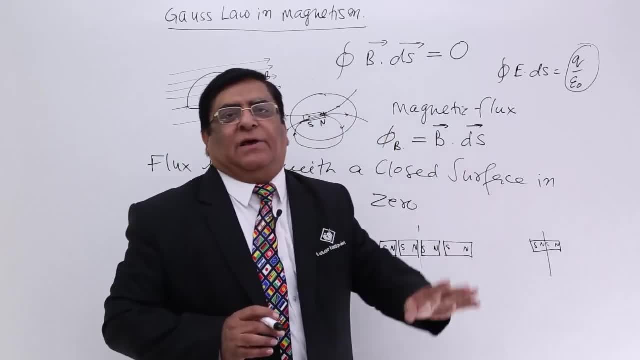 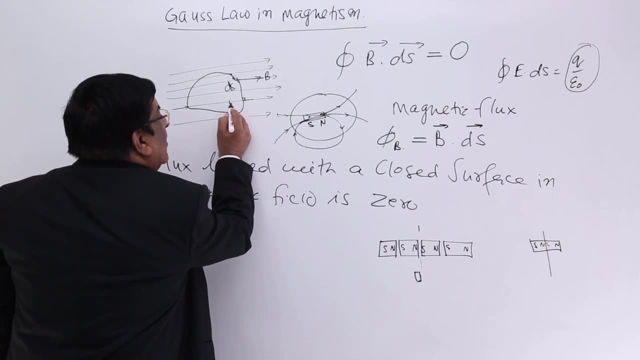 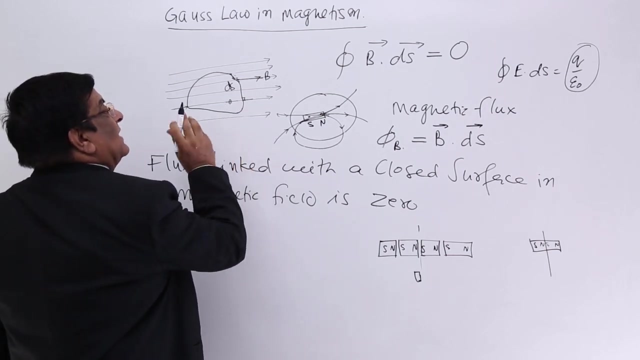 the other side it will appear south pole. So you cannot separate north and south. That means: whatever small is your Gaussian surface, so small Gaussian surface. This is going out, this is going in. so what is the net effect? what is the net number? 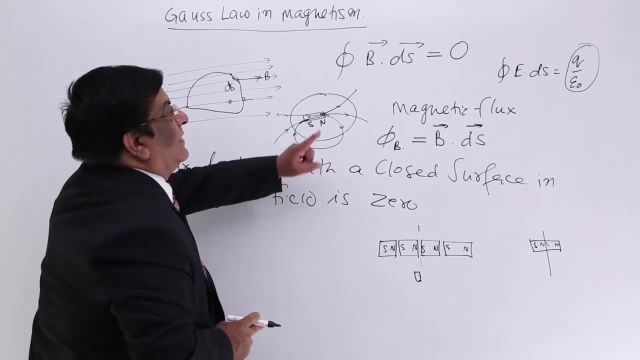 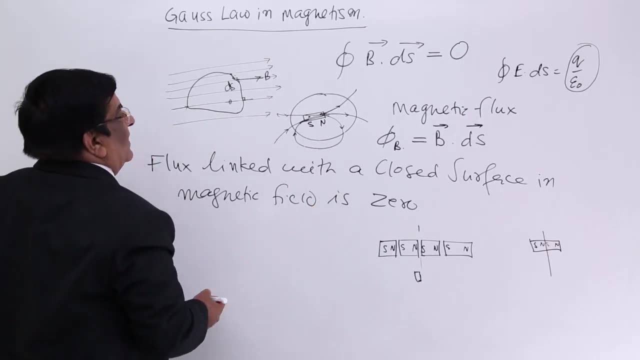 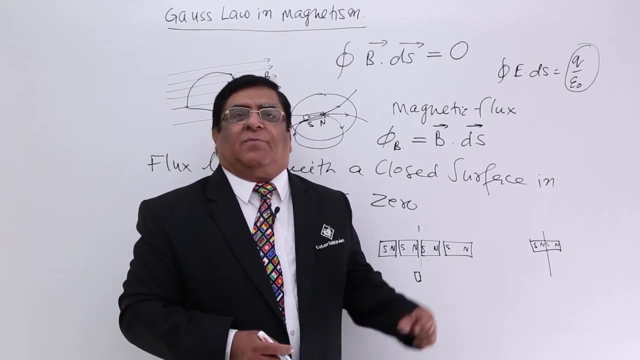 of lines 0. So that is why this is closed. integral Integral BDS is equal to 0.. Please remember this. This is a very, very important thing. This was selected as Maxwell's equation because this tells us about the nature of magnetic. 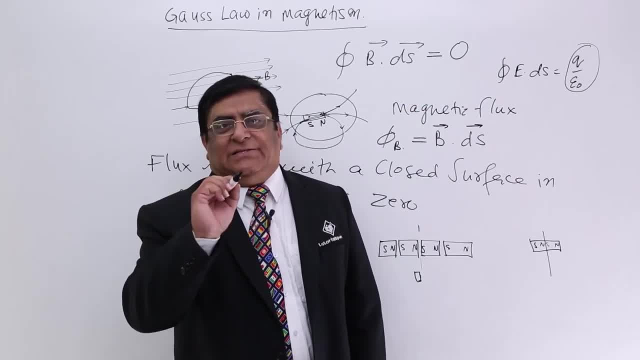 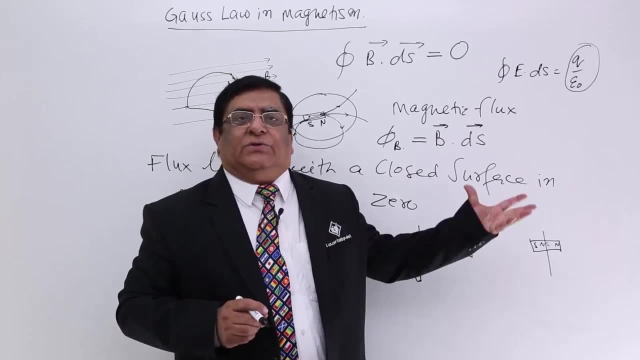 field, That magnetic field, are only continuous lines. They do not have a starting point and they do not have a terminal point. So this is Gauss theorem in magnetization: Even wherever we find the magnetic field, we can find the magnetic field. We can find the magnetic field. 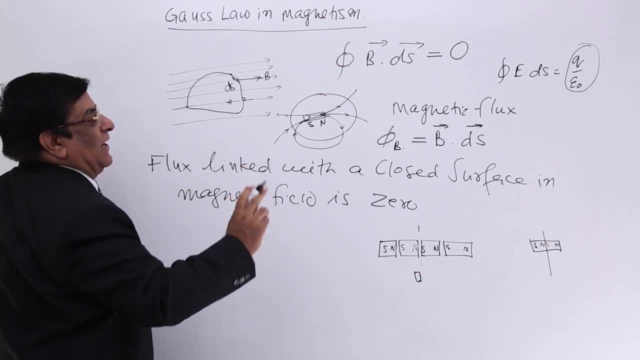 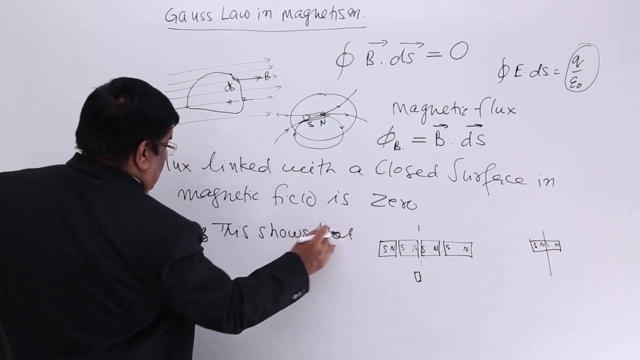 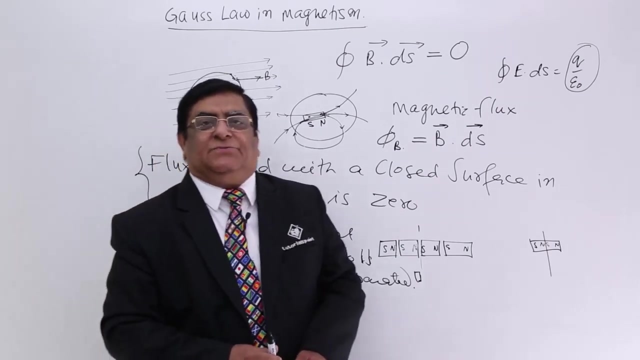 We can find the magnetic field. So if we find the magnetic field, whether for one or two lines, long line, north and south pole, they cannot be separated. So this shows that. So please remember this. So after this you will study certain more properties related to magnetism characteristics. 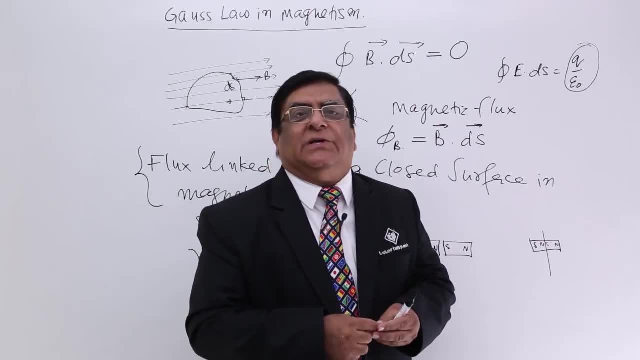 in material, the terms which we are going to use in magnetic calculations in magnetic characteristics. Thank,